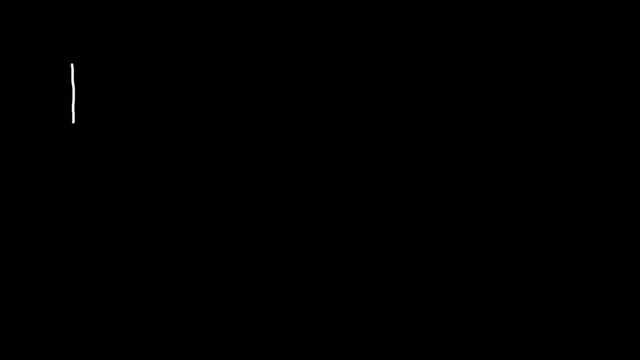 In this video I want to talk about the second law of thermodynamics as it relates to heat, energy and entropy. So let's say, if we have a metal rod placed between a hot object and a cold object, Heat will naturally flow from hot to cold. That's a simple natural process. It's spontaneous, It occurs on its own. 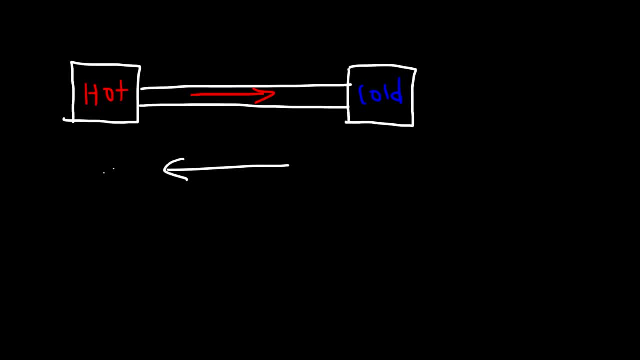 Heat doesn't naturally flow from cold to hot. It just doesn't happen. The only way for you to make it happen is if you were to pump energy into the system. So, for example, a refrigerator will take out heat energy from inside the fridge and 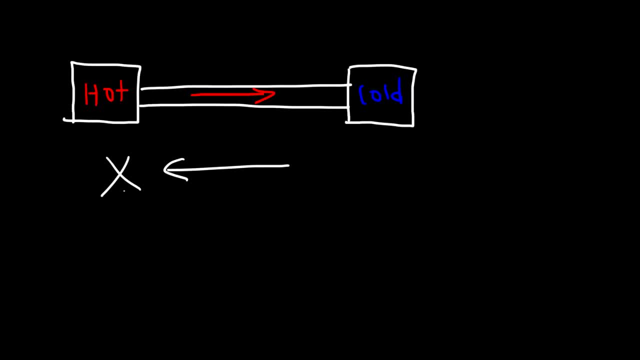 pump it outside of it And that's how a refrigerator can cool this stuff on the inside. But it takes energy to do that. It doesn't happen naturally. A good way to illustrate this is: imagine if, let's say, if you have a ball on top of the hill, The ball will naturally flow in. 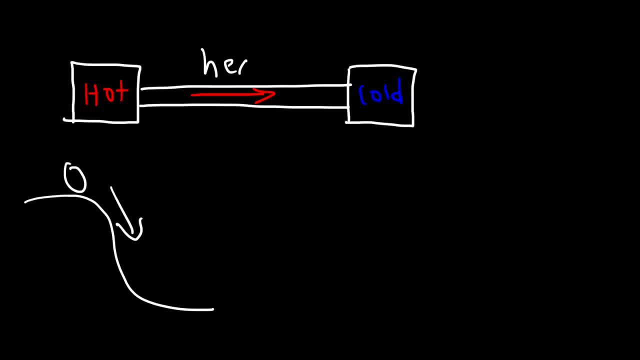 a downward direction. The same way as heat flows from hot to cold, Heat flows from a high temperature, naturally, to a low temperature, And this ball is going to flow from a high position to a low position. Now, if you place the ball at a 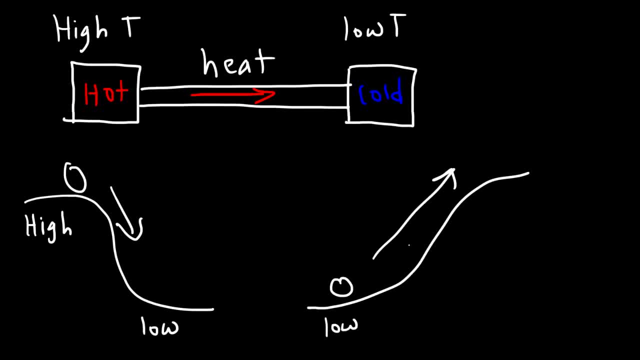 low position. it won't naturally go towards the top. It just doesn't happen. The only way for you to make it happen is you got to put energy into it to get it over that hill, And the same is true for heat. Heat doesn't flow naturally from cold to hot. Now you could make it happen, You can. 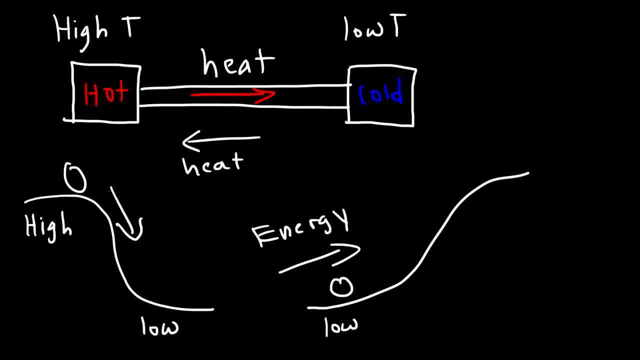 pump heat to warm up a certain environment. Heat pumps do that, However, it costs energy to do so. Now, as heat flows from hot to cold, this is a spontaneous process, And for a spontaneous process, the entropy increases. It's going to be greater than zero, And that's another. 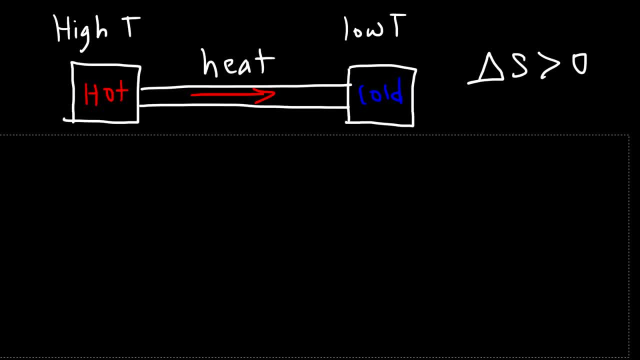 statement of the second law of thermodynamics. For natural processes, the change in entropy will be greater than zero. Now, if you have an ideal reversible process, at best the entropy can be equal to zero. However, most systems do not behave perfectly, So a natural, spontaneous process will tend to lead to.